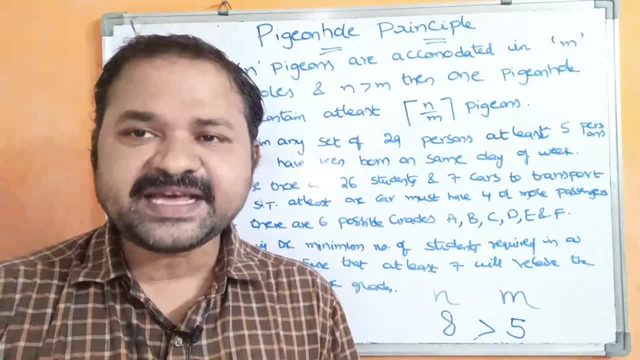 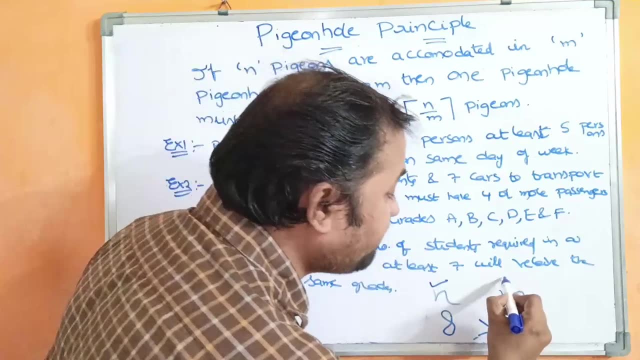 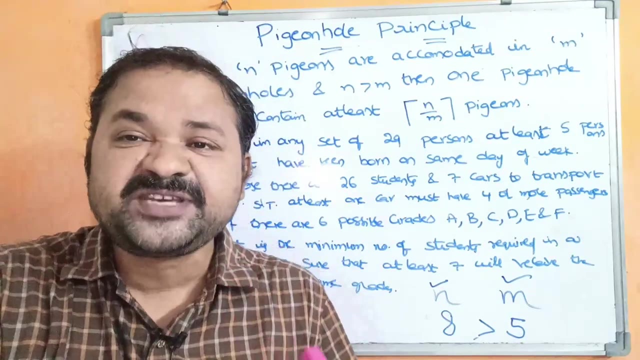 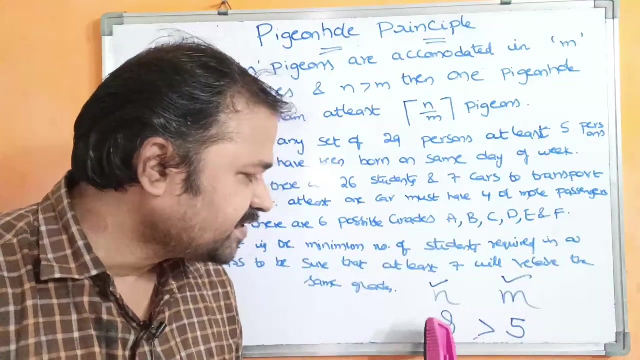 So number of Pigeons must be greater than number of Pigeon holes. Let we have N objects and M containers. So objects are placed in containers, So number of objects should be greater than number of containers. So, just like, just likewise, number of Pigeons must be greater than number of Pigeon. 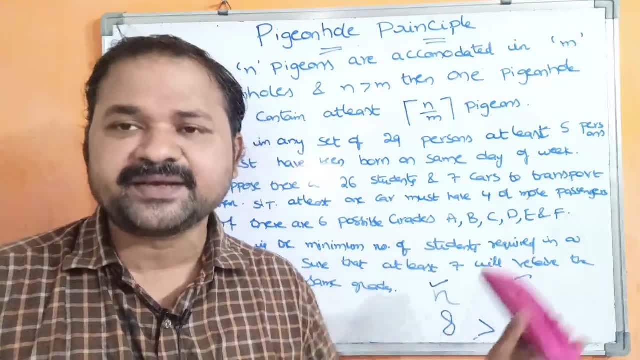 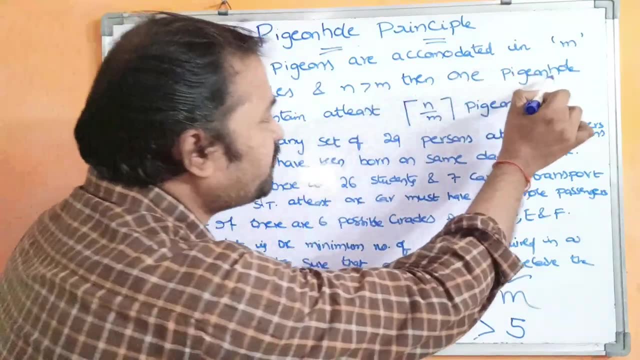 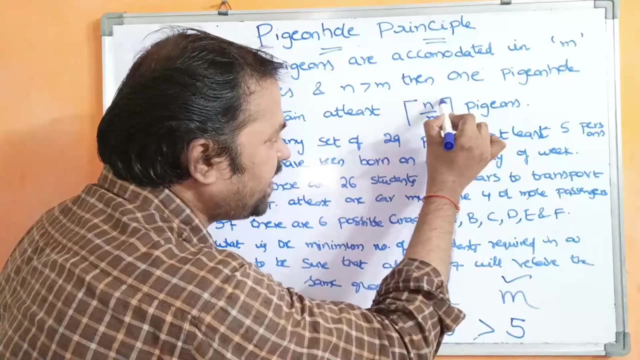 holes. So Pigeons are represented by N, Pigeon holes are represented by M, and N value should be greater than M. Then one Pigeon hole Must contain, at least here. this function is this up arrow. Here we have only upper left. 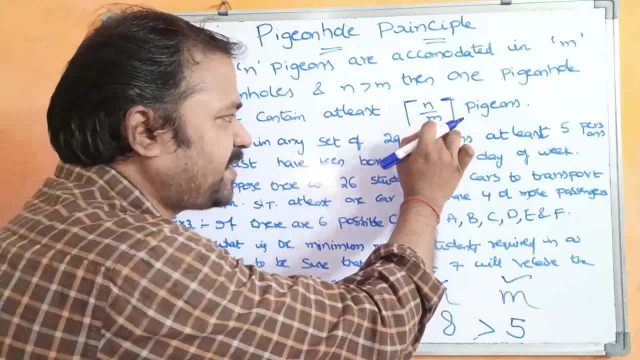 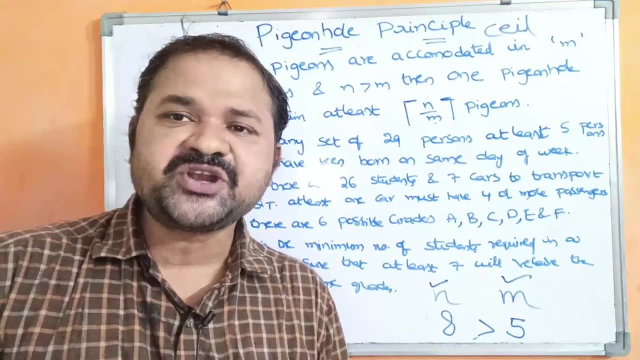 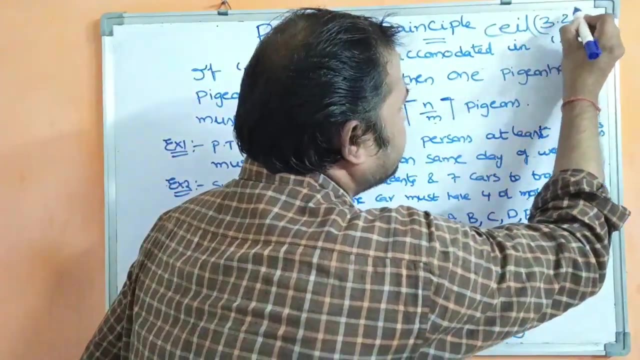 square bracket. We don't have down square brackets. This function is called as seal function. What is seal function? Seal function always produces next integer value. So let we have seal of 3.2.. 3.2 means after 3, what is the next integer value, 4.. 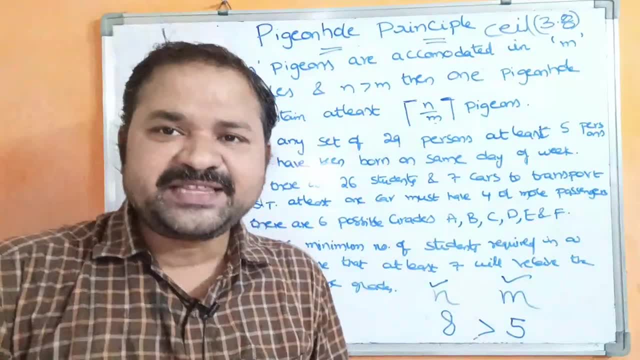 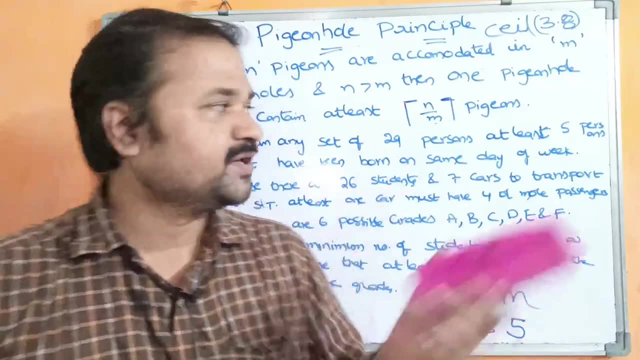 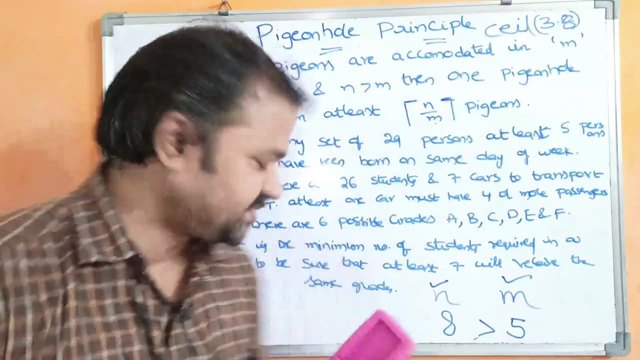 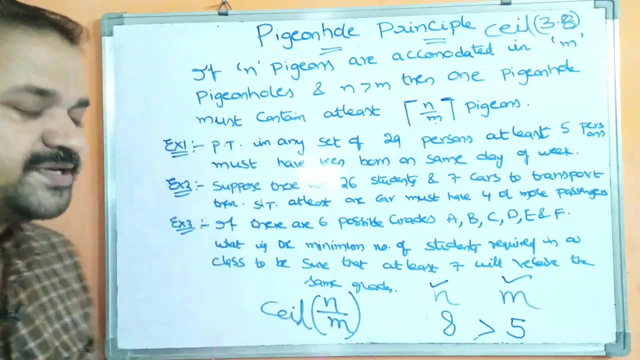 Seal of 3.8.. After 3, what is the next integer value, 4.. So seal function always produces next integer value. So here, what is the problem? here? One Pigeon hole must contain at least N by M Pigeons. So one Pigeon hole must contain at least seal of N by M Pigeons. So this is: 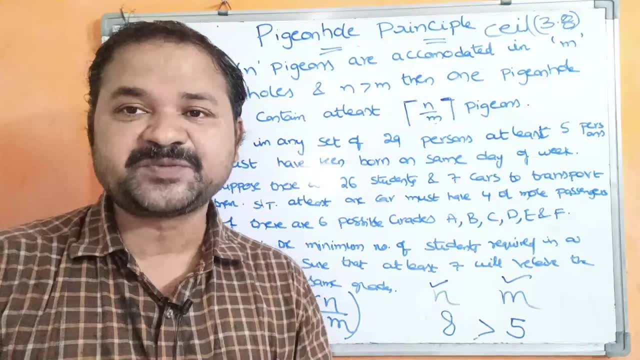 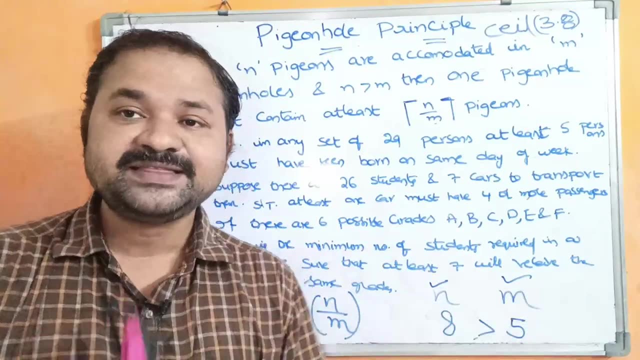 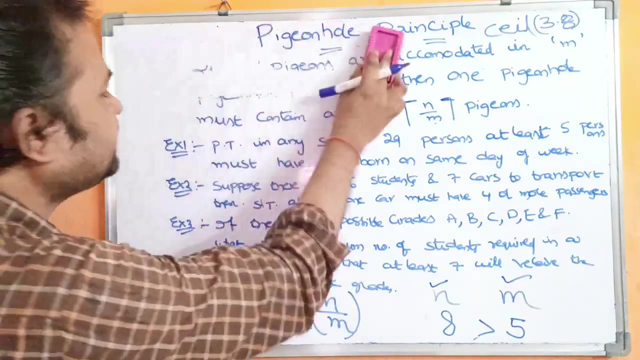 the problem. This is about what is Pigeon hole principle. Let we have Now N Pigeons and M Pigeon holes and N is greater than M, Then at least one Pigeon hole must contain seal of N by M Pigeons. Now let us solve these three examples. So for space, 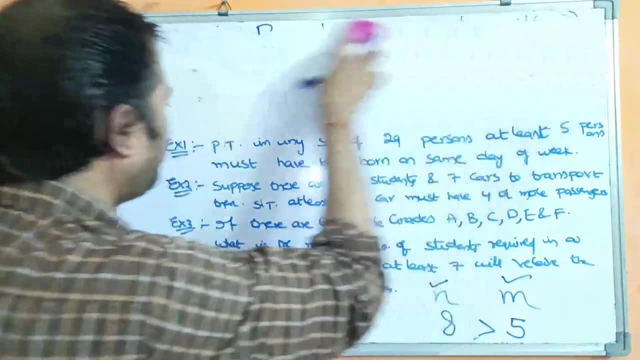 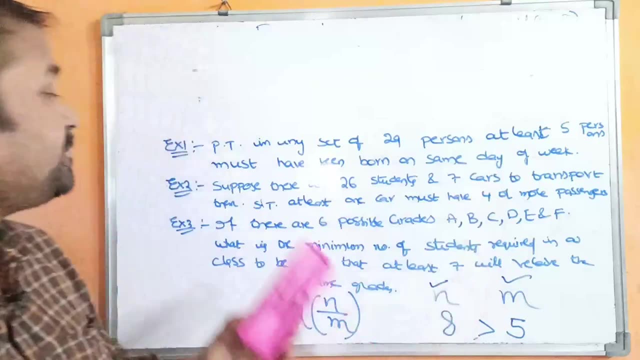 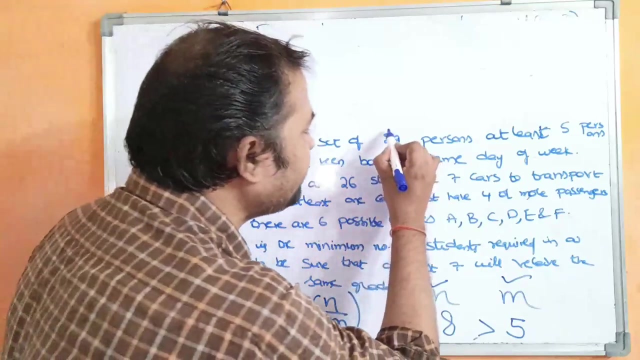 constraints, I am erasing this portion. Let us see the first problem. Prove that in any set of 29 persons, at least 5 persons must have been born on the same day of the week. So how many persons are given? 29 persons are given Here. number of persons. 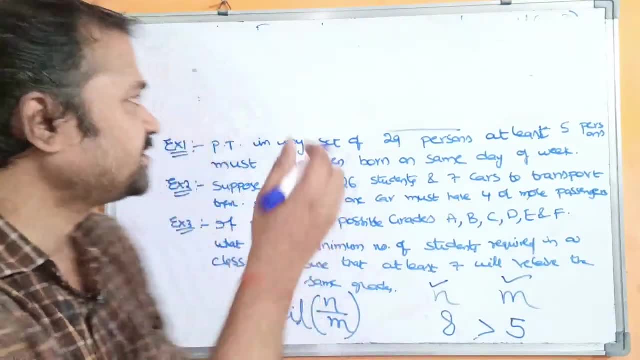 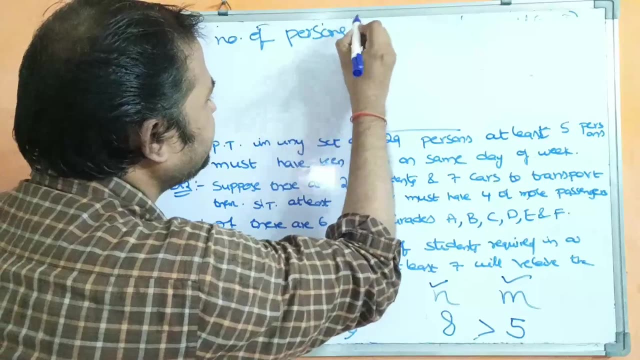 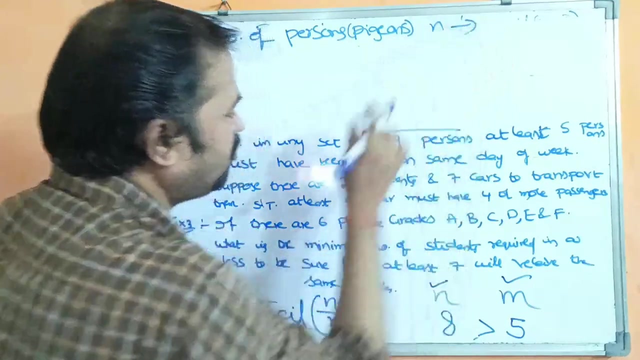 are nothing but 29.. Persons are nothing but Pigeons. Okay, So number of persons, Number of persons. So number of persons means Pigeons. So it is denoted by N? N. So what is how many persons are given? 29 persons. 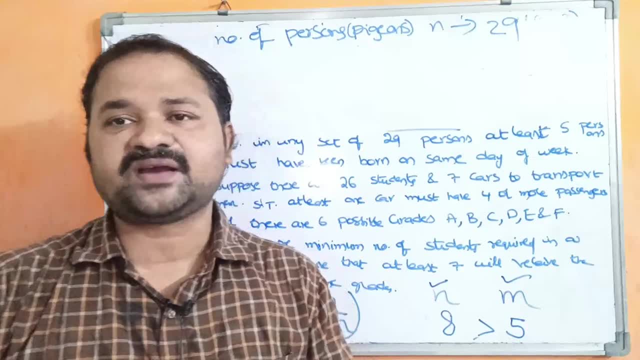 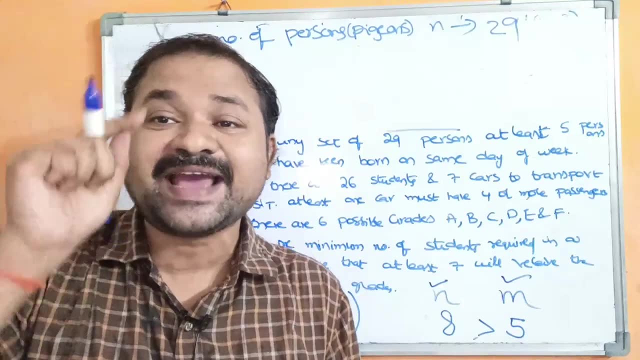 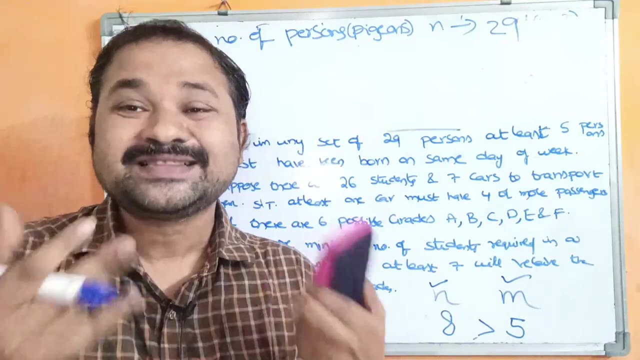 So how many persons must have been born on the same day of the week? So we have to prove that out of 29 persons, at least 5 persons. So we have to prove the result as 5 out of 29 persons. We have to prove 5 persons must have been born on the same day of the week. 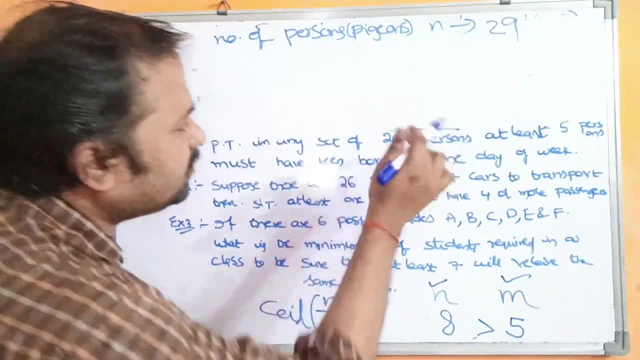 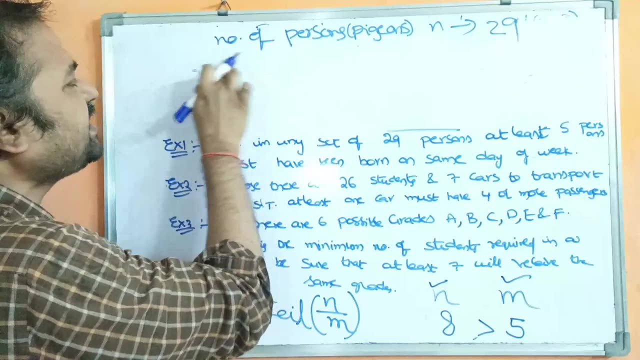 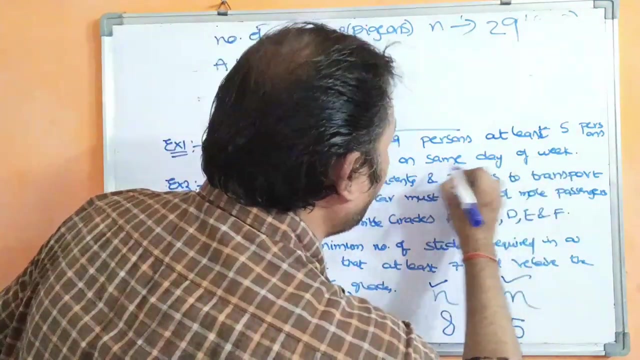 Okay, So here a week. okay, totally, 29 persons are given, So we have to prove the result as 5.. Okay, Okay, So a week will contain how many days? A week contains 7 days. Must born on the same day. 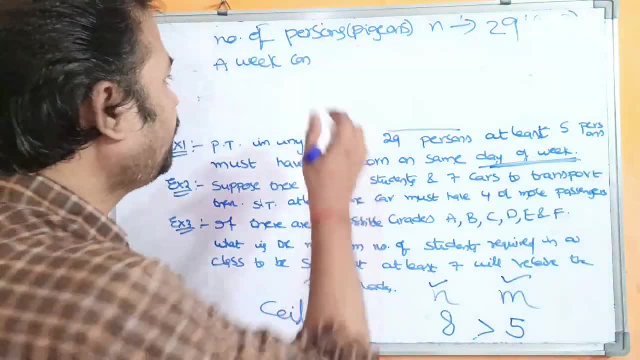 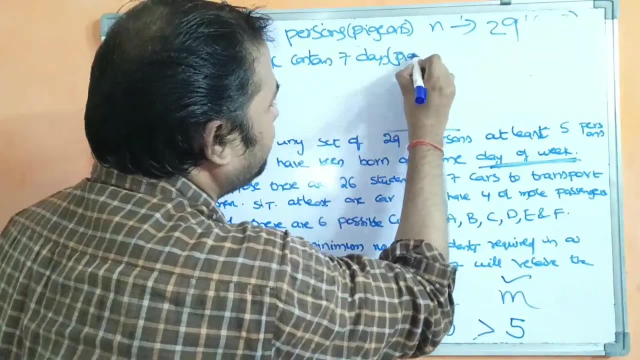 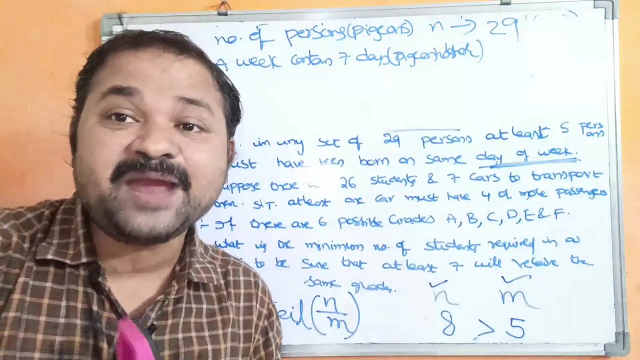 of the week On the same day of the week. So a week contains how many days? 7 days. So these 7 days are nothing but Pigeon holds. Pigeon holds Why? Because we have to prove that 5 persons must born on the same day of the week. Week, week is given. So a week totally. 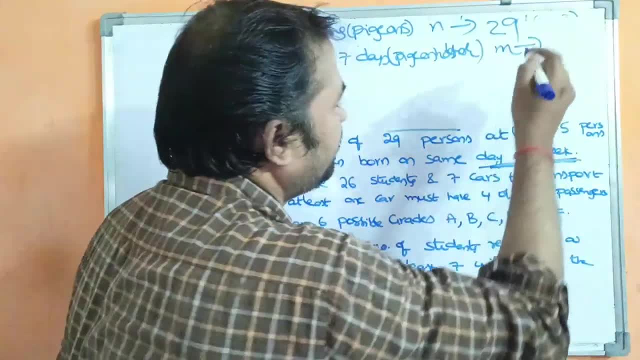 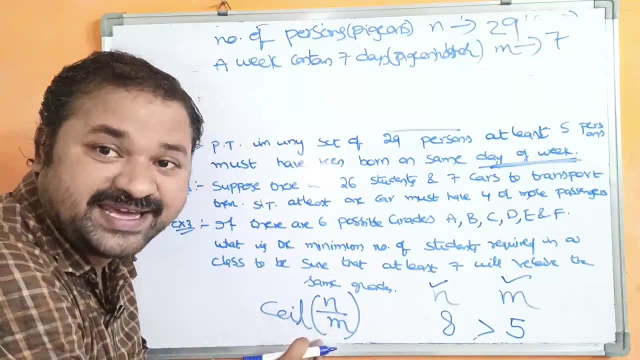 contains 7 days. So this is nothing but M value. So what is M value 7.. What is the result here? At least one Pigeon hold must contain C. law of N by M C. law of N by M C. 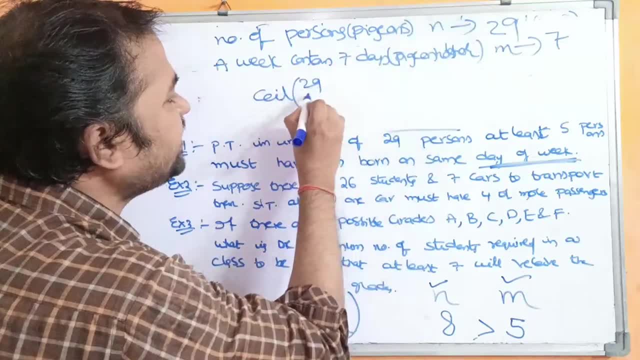 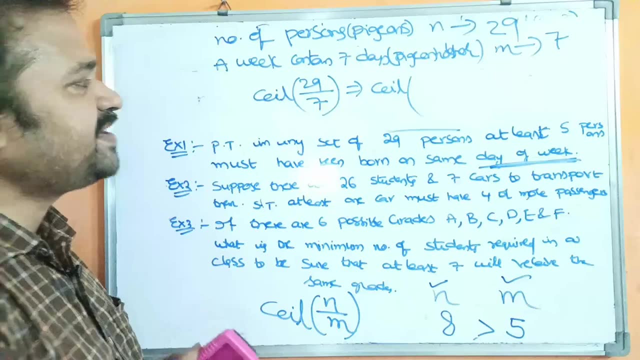 law of what is N. N is given as 29 by what is M, 7.. So that is equal to C law of what is the result of 29 by 7?. So 4 point. So 7, fourths are 29.. Next to 4 point, So that is. 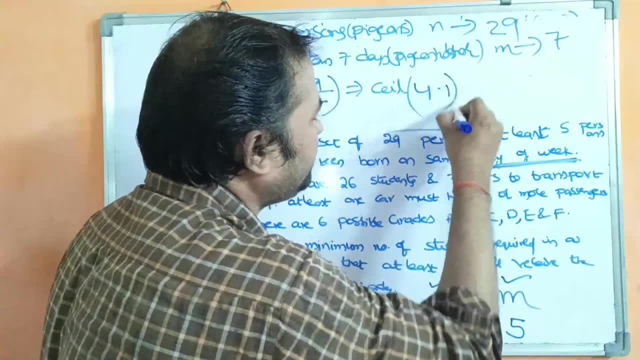 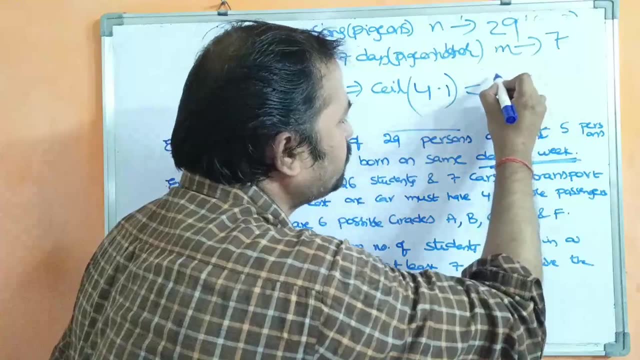 2. So we will get 1.. So 7 1s. So C law of 4 point 1.. We will get C law of 4 point 1, something. So C law of 4 point 1 means what It will gives the next integer value After 4. we will. 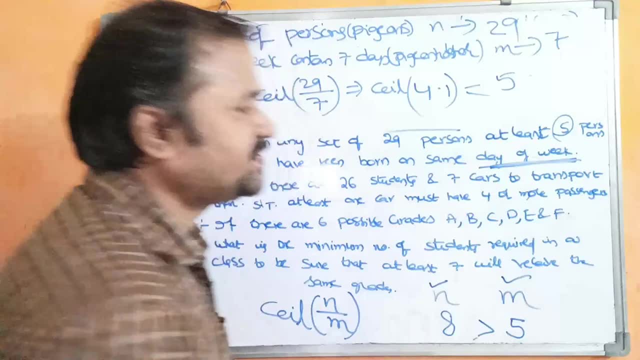 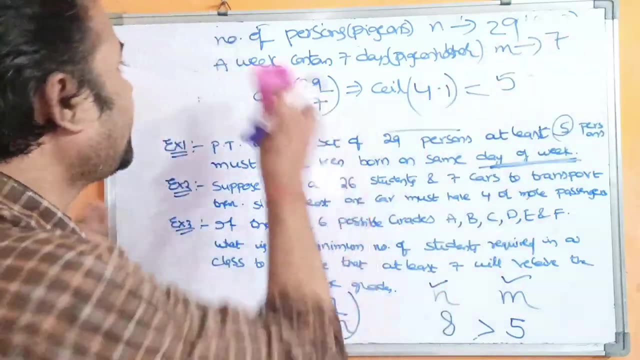 have 5.. So we have to prove that 5 as the result. So we can conclude that 5 persons must born on the same day of the week. So in this way we can do the problem. Now let us see the second problem. Let us see what is the second problem. Suppose there are 26. 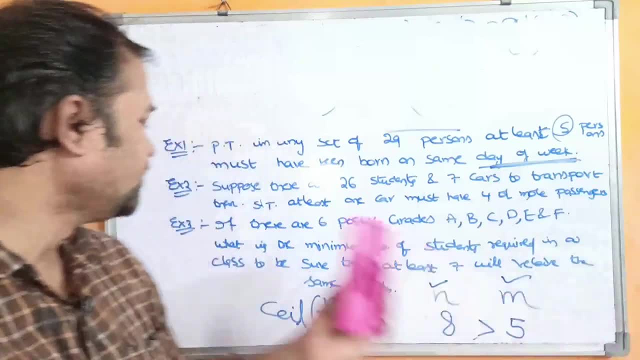 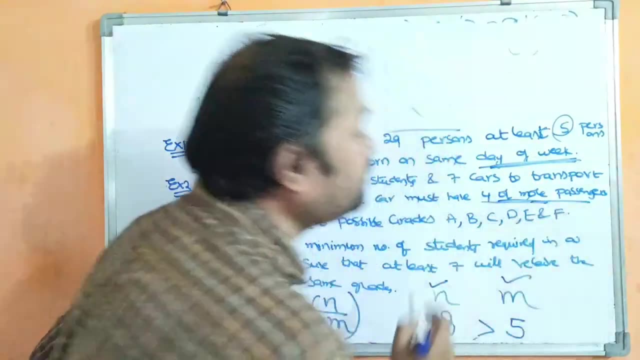 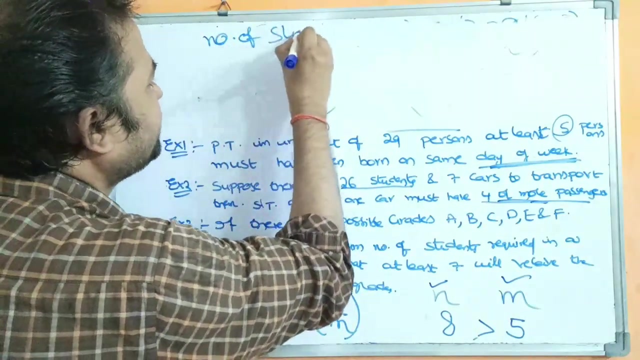 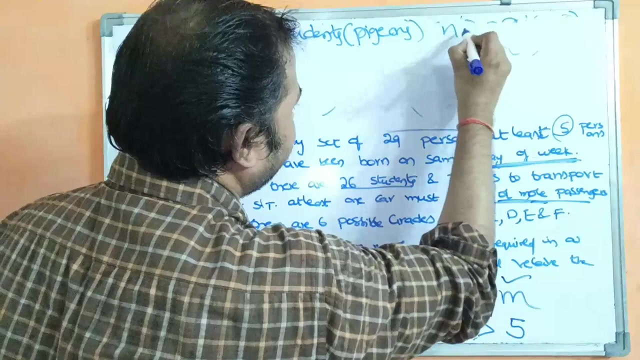 students And 7 cars to transport them, So that at least one car must have 4 or more passengers. So number of students are 26.. So number of students, So number of students are nothing but number of Pigeons. So Pigeons are represented by N. So how many students are there? 26 students. 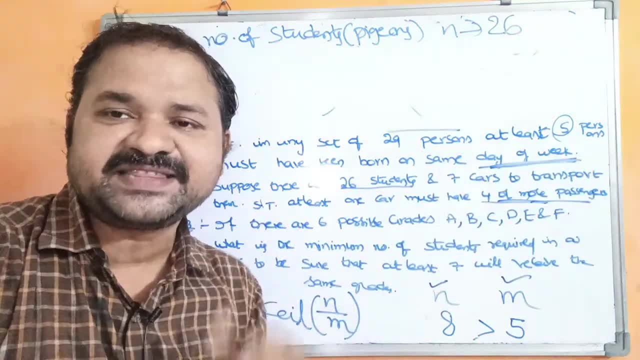 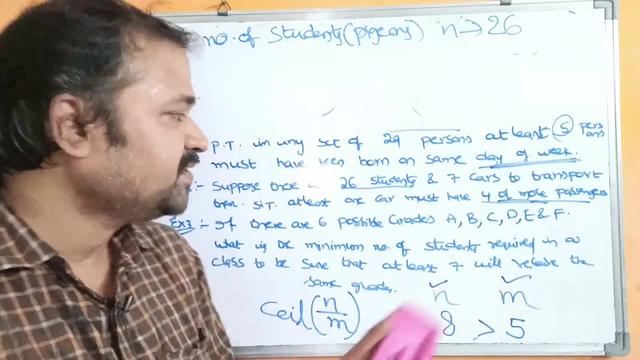 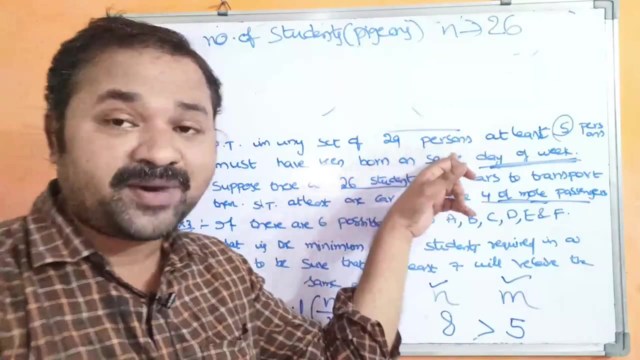 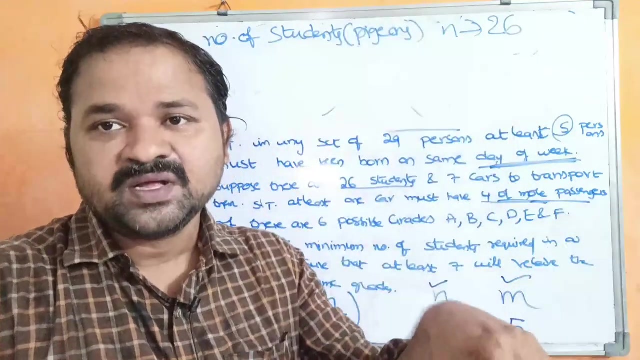 And to transport them. so 7 is nothing but what number of pgm poles? why? because we know that n value should be greater than m, so n is 26. 26 is greater than 7. in the previous example also, number of persons are 29 and a v contains 7, so n should be greater than m. so n value should be 29. because 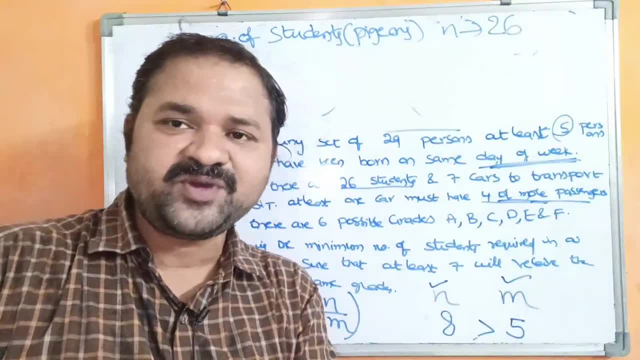 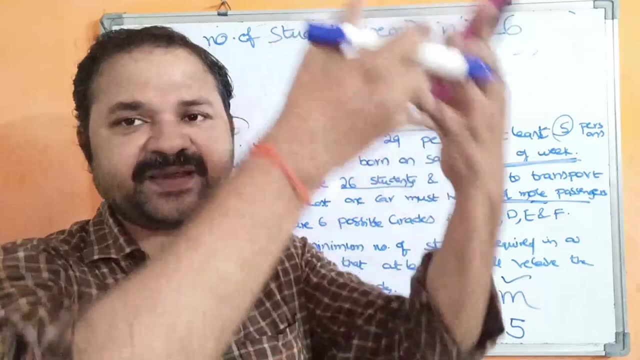 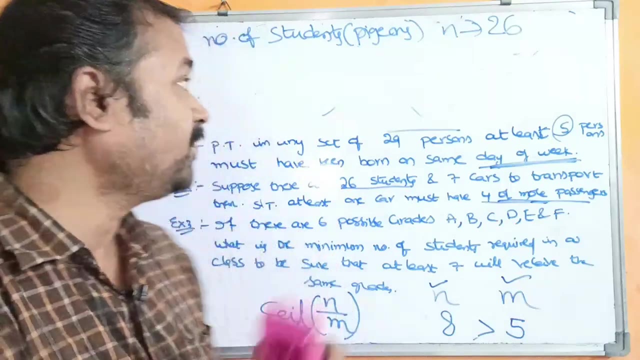 that is bigger value. m value should be 7. why? because that is the smaller value. in the second problem also, n value is 26, m value is 7. because 26 is bigger value, 7 is smaller value because in the problem only that we have specified as n is greater than m. okay, and number of cars. so how? 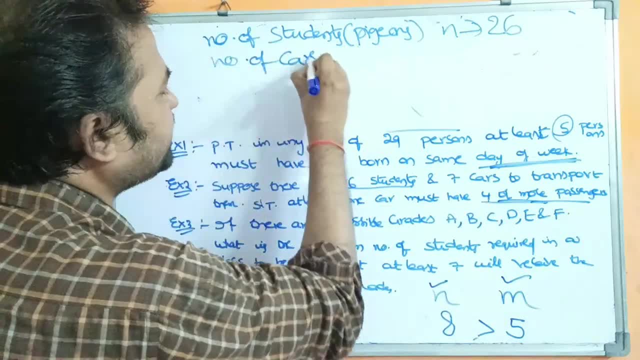 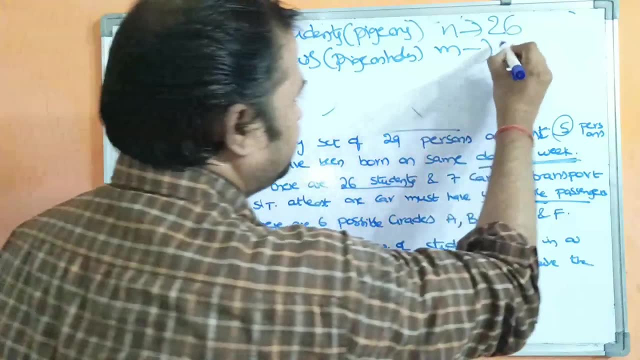 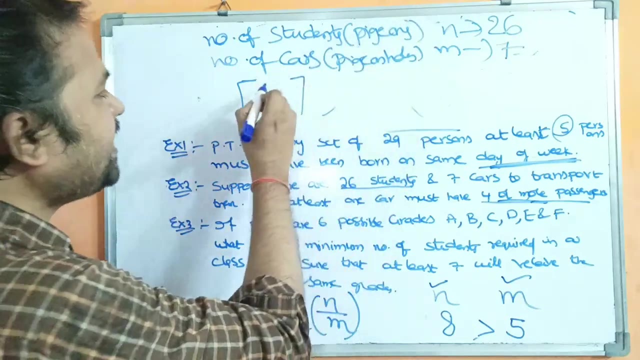 many cars are there? number of cars are nothing but what pgm holes? why? because it is smaller value. so m is equal to 7, 7. so what is the formula here? at least one pgm hole must contain n by m. what is n? 26 by. 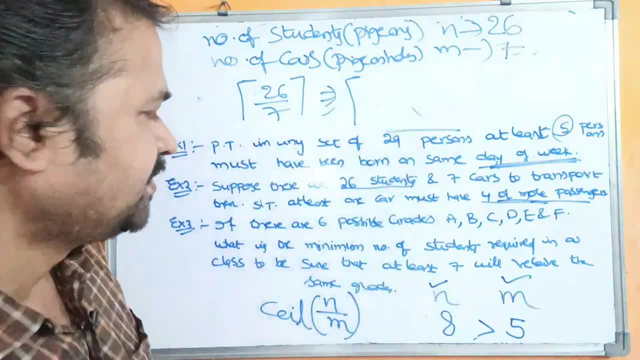 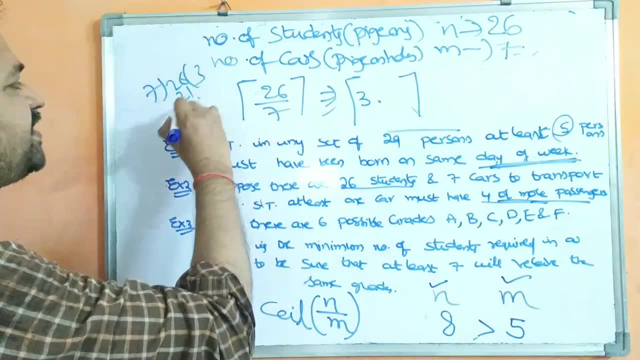 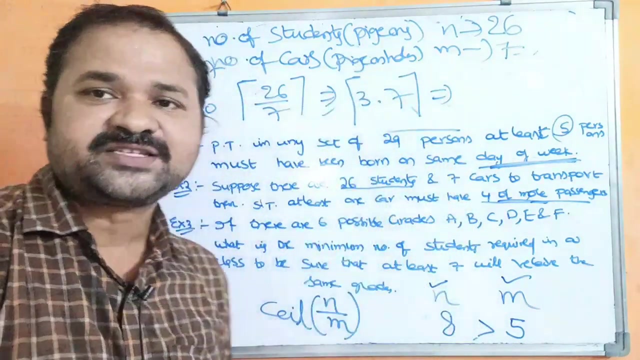 7. what is the result of 26 by 7? 26 by 7, so 7. threes are 21, so 7. 26. 7 threes are 21, 5.77, so 3.7, something. so this is nothing but seal function. seal means it always produces next integer. 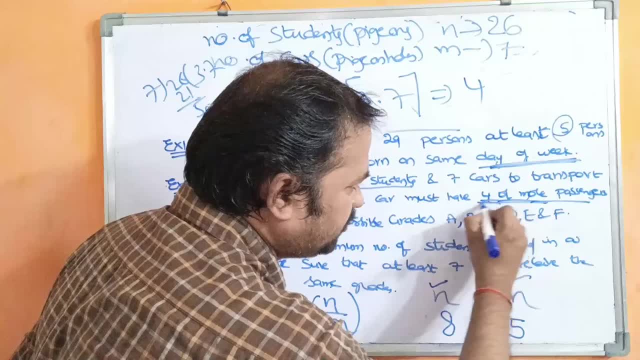 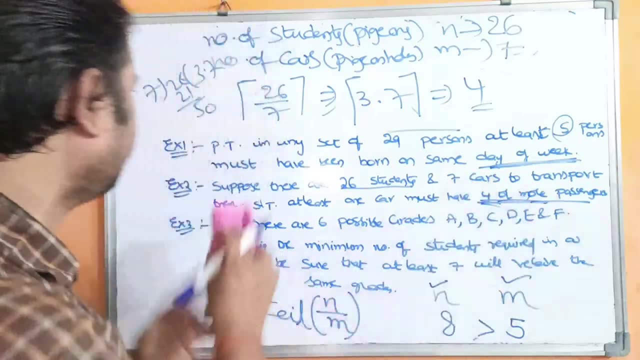 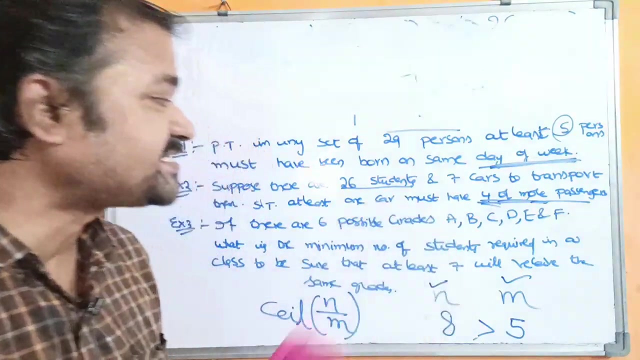 value. the next integer value is 4. here we have to prove that four or more passengers, so we got the result as 4. so with this we can conclude that the solution is correct. now let us see the third example. if there are six possible grades- a, b, c, d, e, f- what is the minimum number of students?